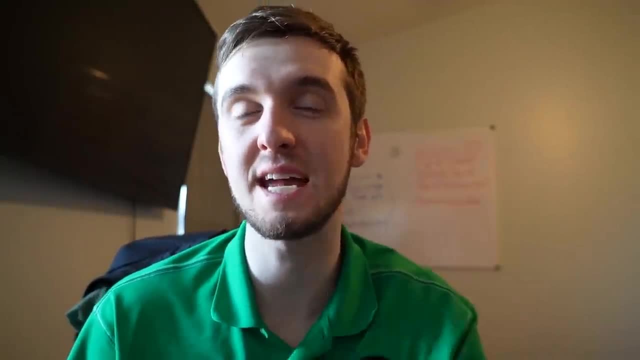 What's up house fans? It's me Packy, and today I'm doing part two of making an illegal bowling ball. I got this brand new DV8 collision here. I'm going to make it illegal, but how I'm going to make it. 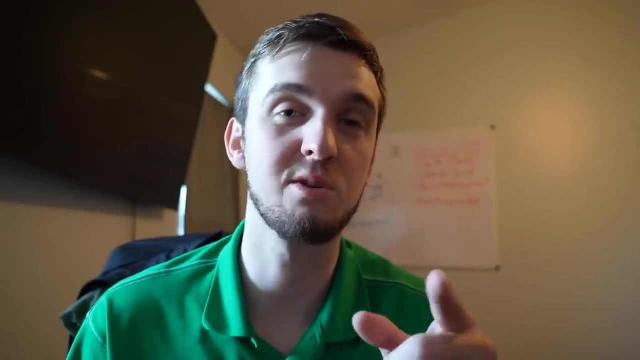 illegal. you guys will have to find out once I take it back to the drill room. So I will see you guys down at the Shocker Sports Grill and Lanes right about. hold on, hold on. but first but first, you guys know what to do. Just hit that subscribe button down below. 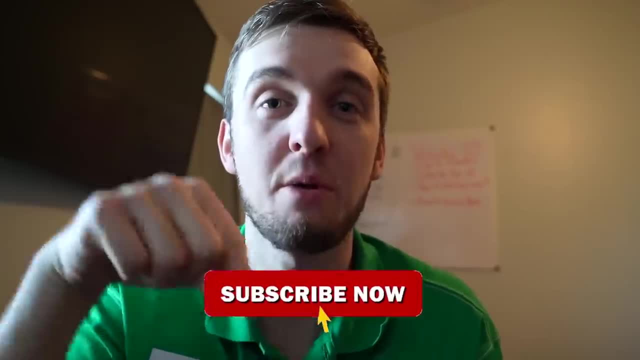 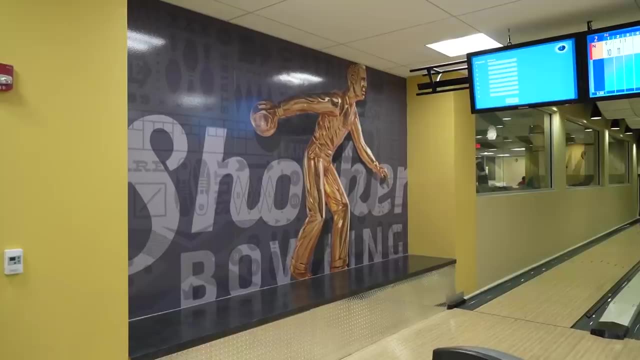 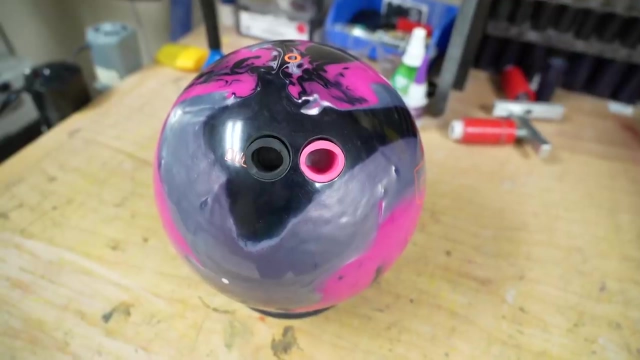 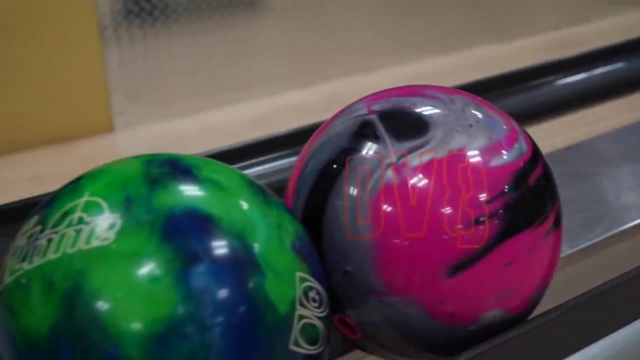 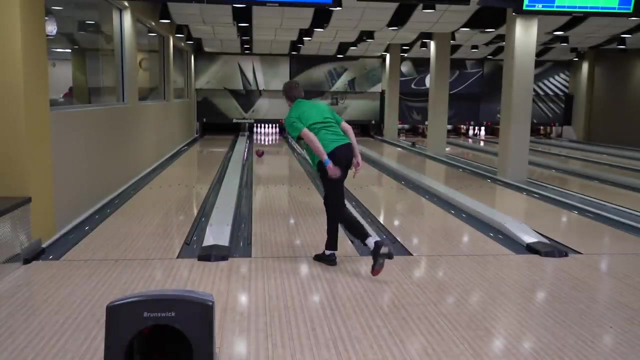 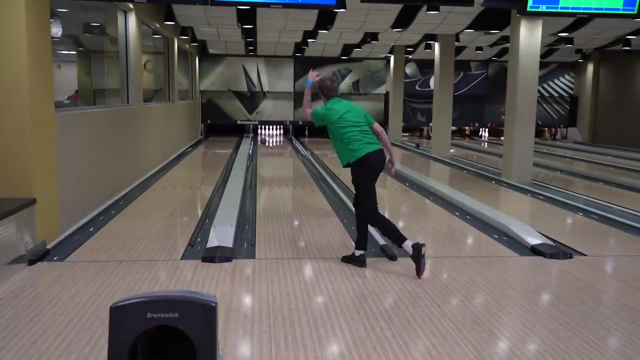 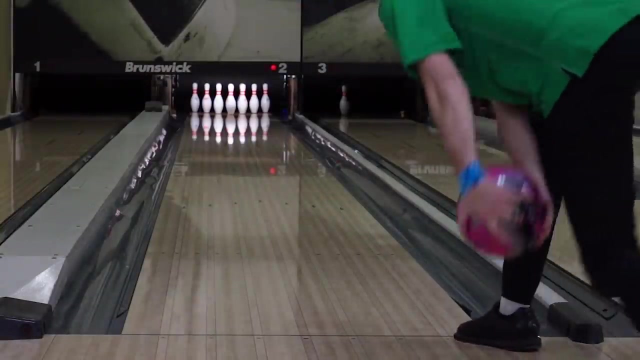 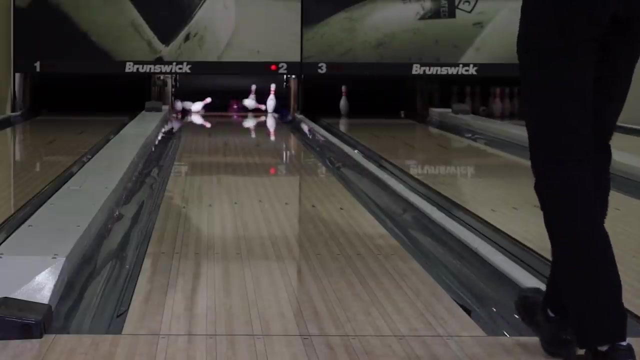 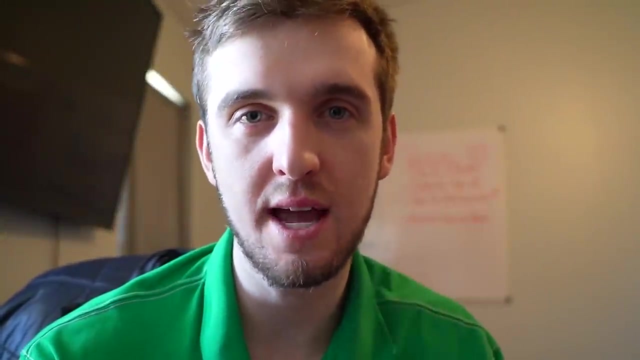 down below. just hit that subscribe button down below to follow along for more videos like this and more PBA tournament vlogs, And we're out, All right. So I've drilled it with a normal dual angle layout set up And I'm going to go ahead and do a little bit of a drill. So I'm going to go ahead and do. 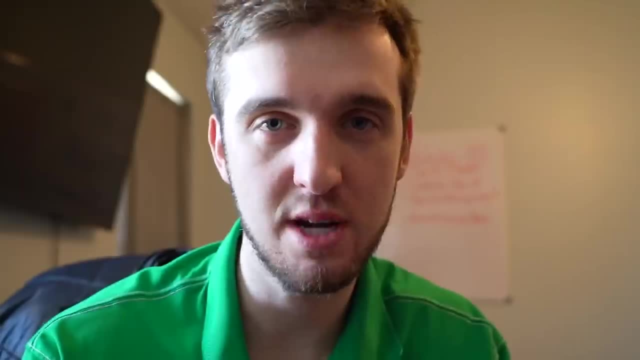 a little bit of a drill. So I'm going to go ahead and do a little bit of a drill. So I'm going to go 60 degrees by four and three quarters by 65 degree layout. I'm now going to take it down to: 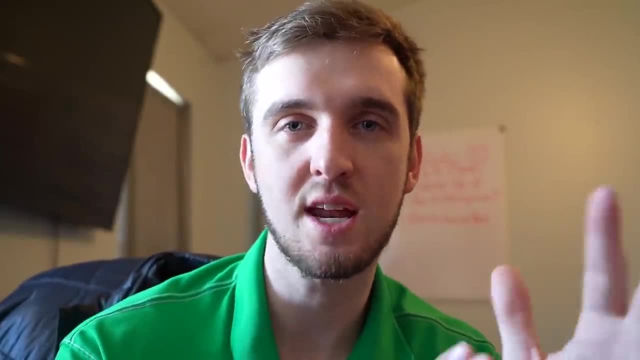 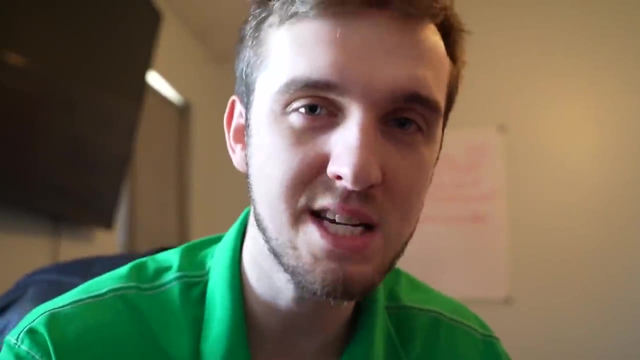 the lanes bowl one game with it. show you guys that normal reaction that it gives me. And then I'm going to take it back to the drill room, make this thing so illegal you guys won't even be able to believe it. And then I'm going to take it back to the lanes and show you guys why it's illegal. 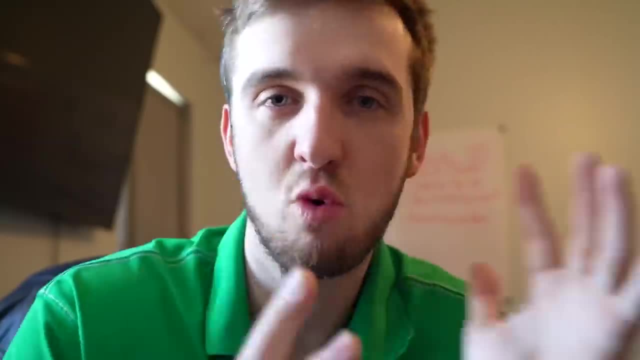 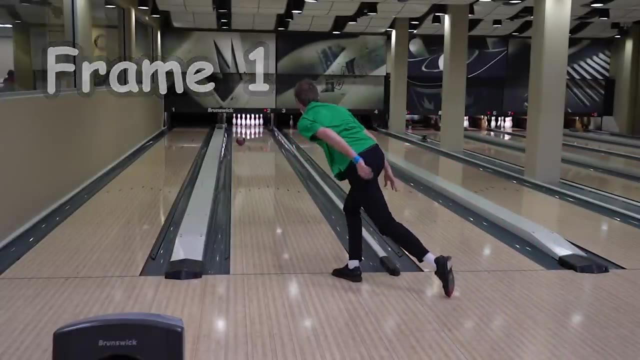 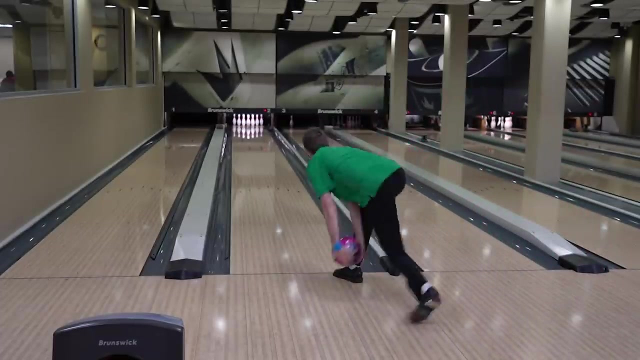 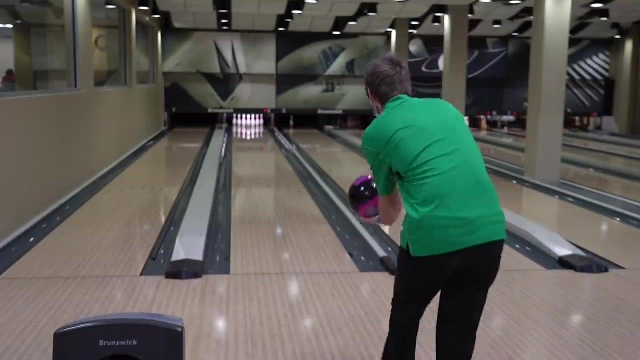 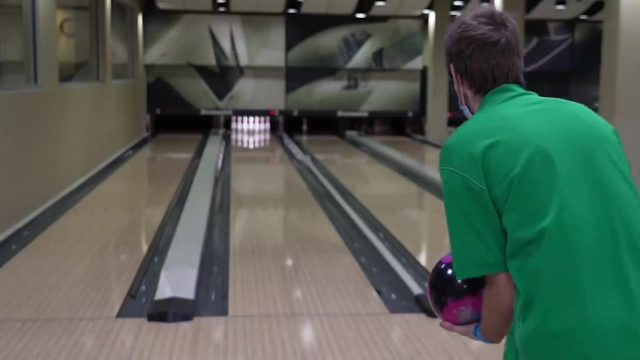 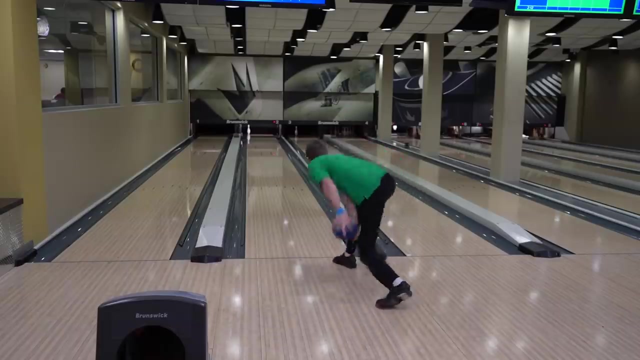 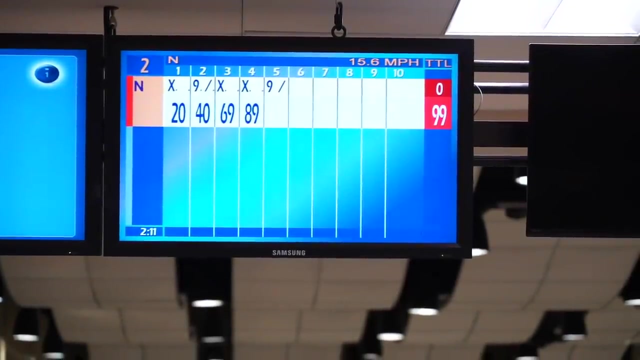 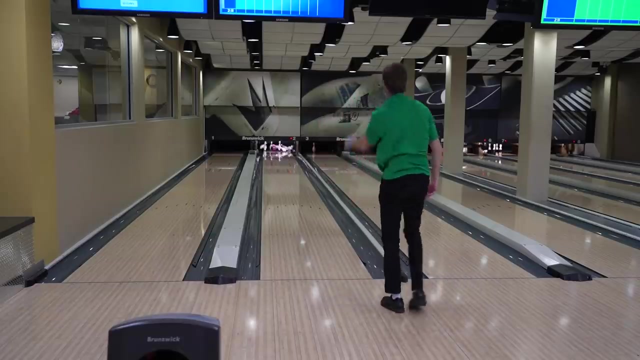 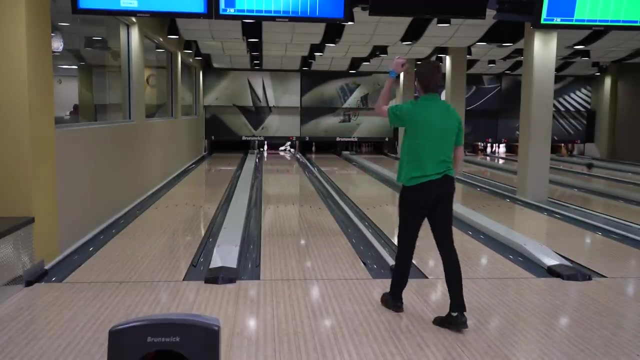 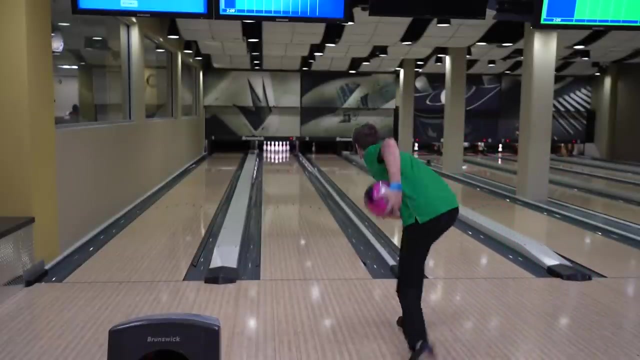 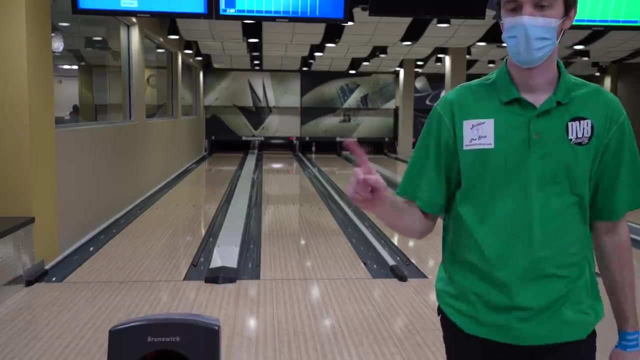 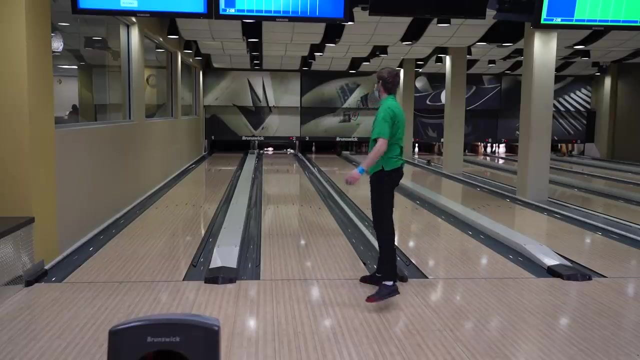 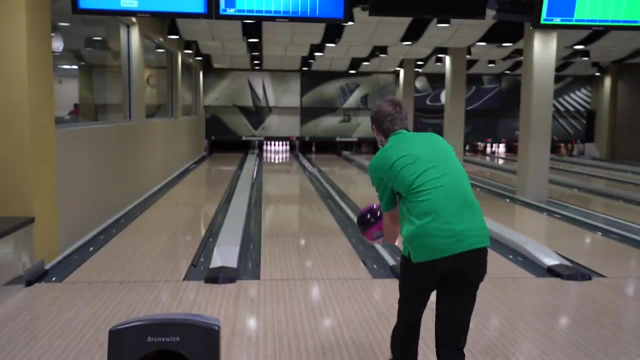 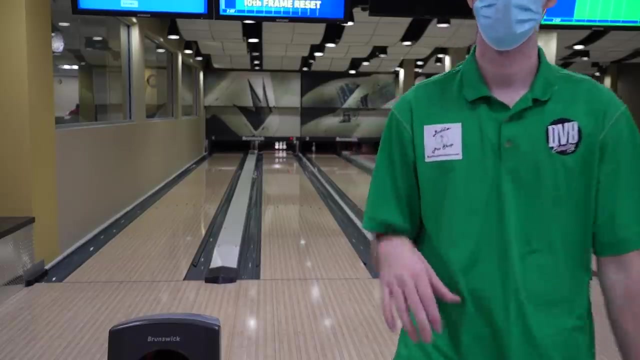 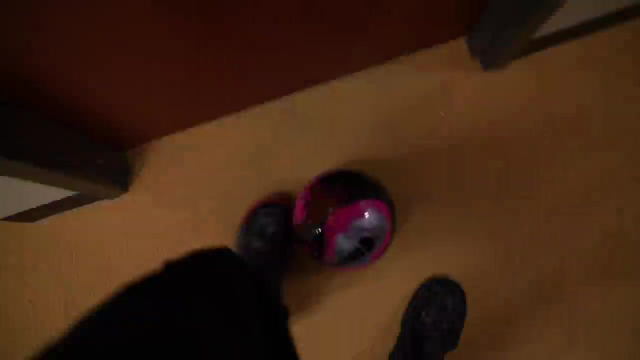 and why they changed the rule a little bit, and what rule they changed. And now let's go to the lanes. And now let's go to the lanes, Let's go, Let's go, Let's go. There's obviously no professional when it comes to being in the pro shop. 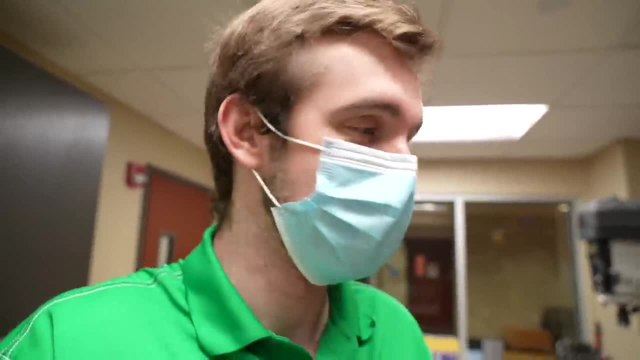 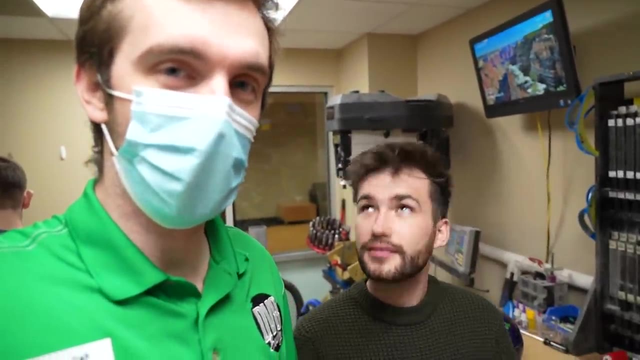 I basically know how to throw two finger holes in the ball, and that's it. Same. Same with Sloan, even though he owns a pro shop. So, Sloan, Yes sir. Now let me have you here. Why are weight holes actually illegal? 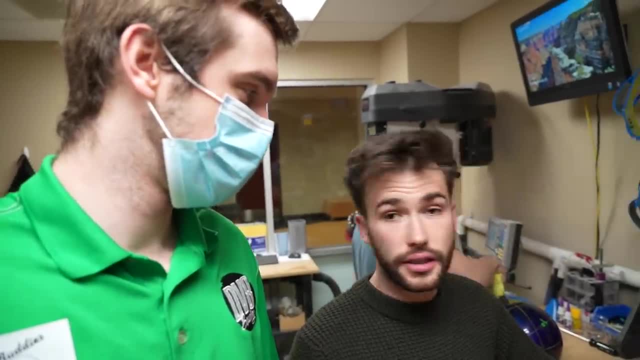 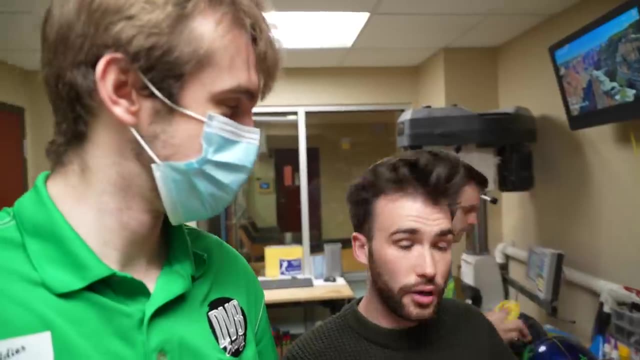 I know they changed the rule like two years ago. There's a variety of different reasons, because obviously you can change the shape. My hair looks terrible, It's okay, Mine always looks terrible. There you go, There we go. You can change the shape and the ball reaction based off where you put the extra hole. 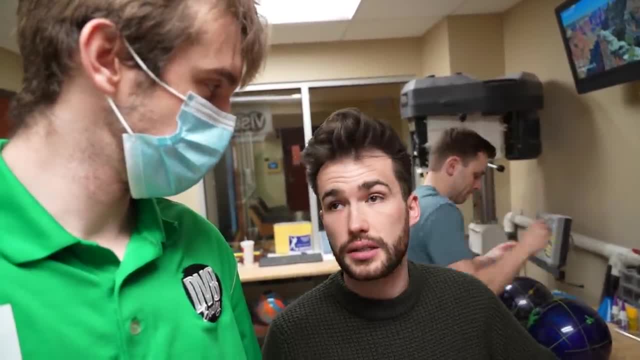 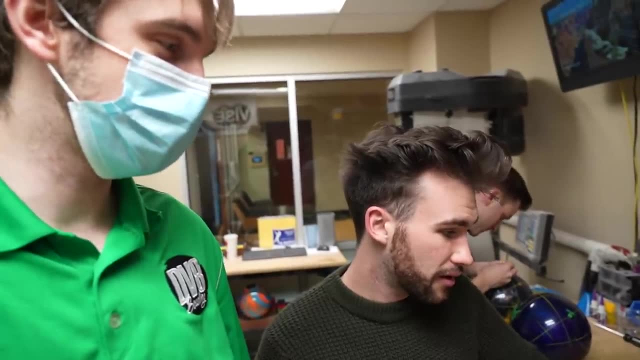 So there's a couple of different positions that you can put, So weight holes depending on size, depth, that will manipulate the ball roll. I want to make this the most illegal, So I'm going to put a big- so you're saying big hole deep. 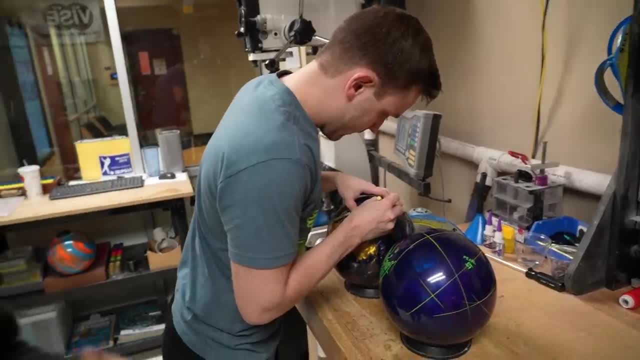 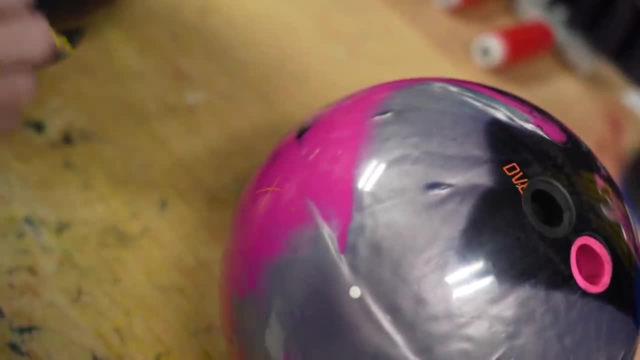 I mean deep big hole? yeah, pretty much. Mark, with a pencil where I should put the weight hole, Just throw it on there. That's not far away. It's pretty low but we like it. That's not far away. 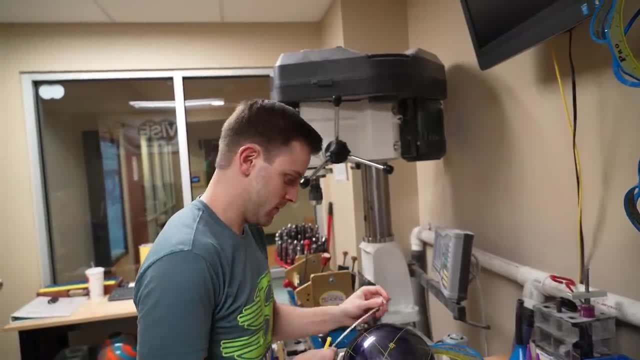 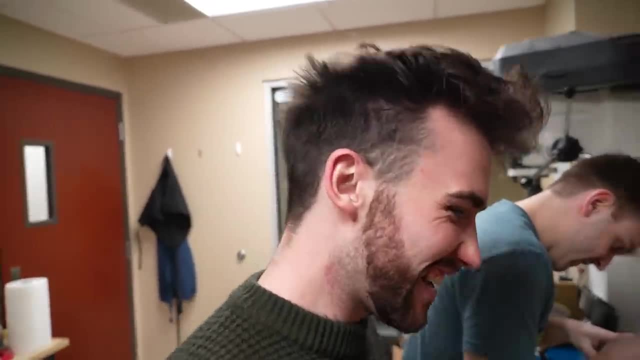 It's a good guess. How much more is it going to hook now? Miles Like three, Three to seven boards maximum. I wasn't sure what the measurement was going to be. I was going to say Three to seven. Yeah, three to seven. 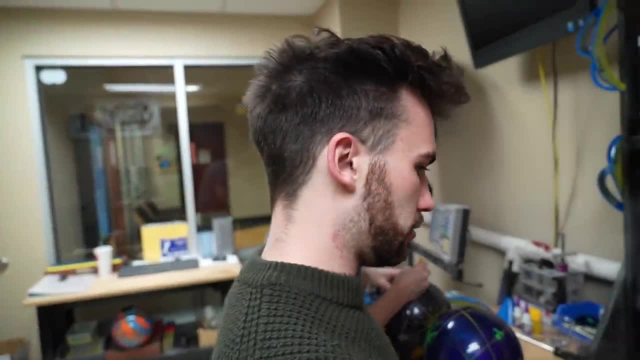 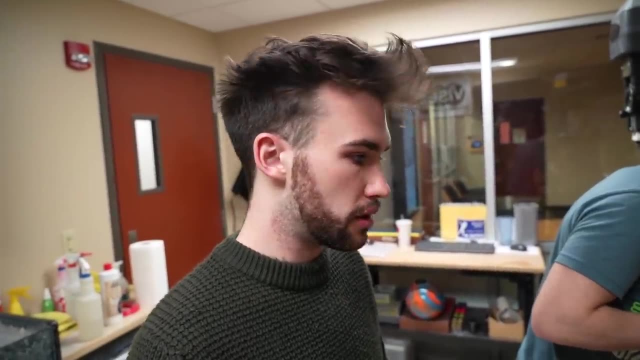 I don't know. So, yeah, just go with. so, obviously, the biggest bit that you can put in it. Inch and a quarter. Yeah, On tour it was an inch and three eighths. Everything else was an inch and a quarter previously, but I believe on the PBA you could. 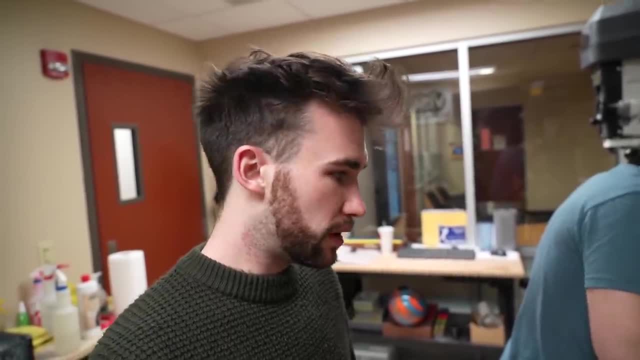 use an inch and three eighths. So inch and three eighths as deep as I can, Only on the PBA And since you're a PBA player, Inch and three eighths, I'll allow it All the way in. 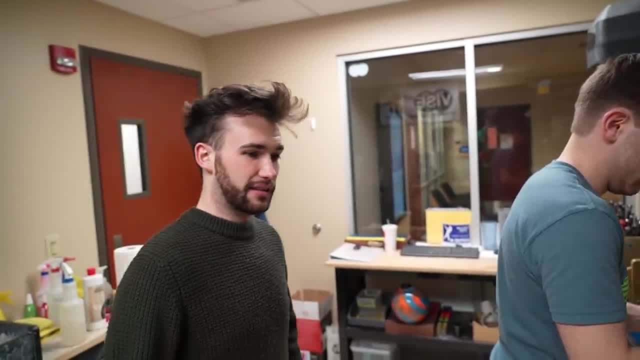 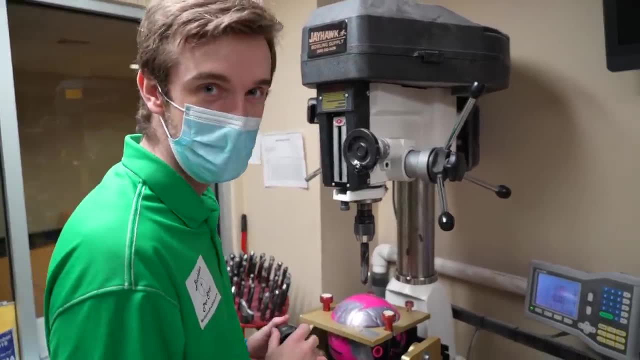 Yeah, Inch and three eighths and just go like two and a half deep. All right, So we went with an inch and a quarter, because USB-C regulations inch and a quarter. We'll stick to that Inch and a quarter. 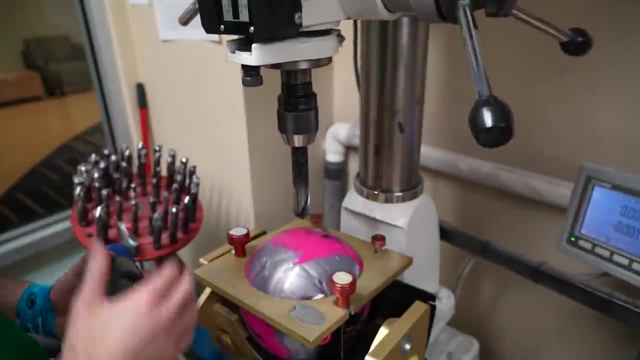 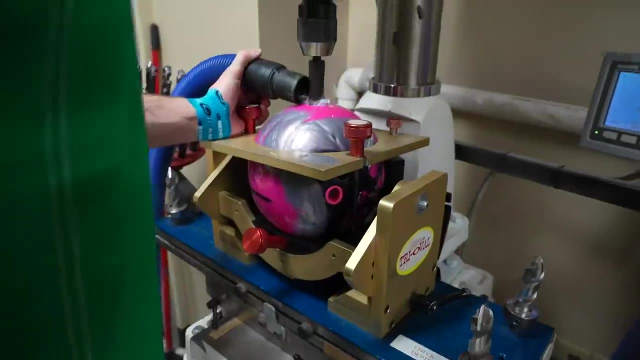 Two inches deep. Three to seven boards more per Chris Sloan, And this is where it's going. I don't know where that is in relation to my pap Frankie just put it on the ball and he's an expert ball driller. It'd be zero. 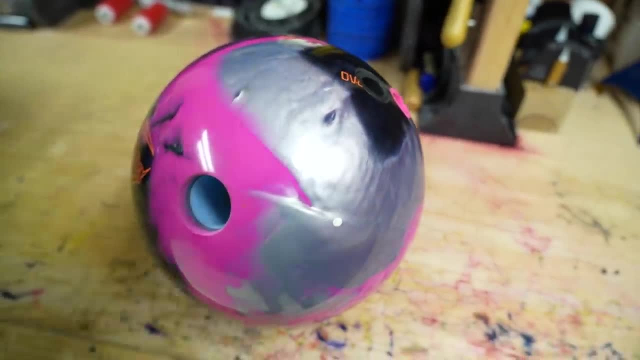 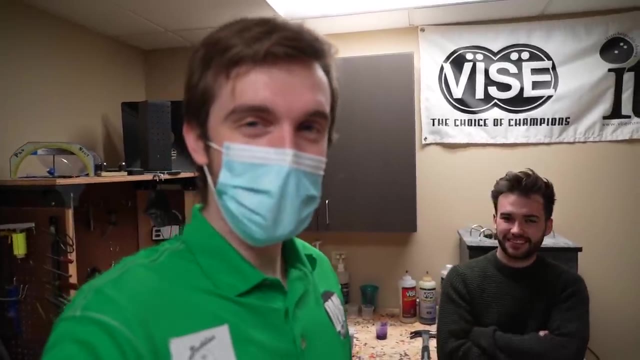 There's days when I just can't fucking make one, Like yesterday. Sloan, You walked that performance, Yeah, Okay. Well, I shot 260 game one. If I shot 260 game one, what am I shooting? Game two: 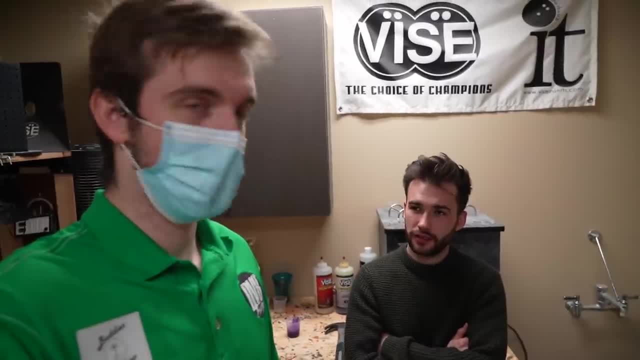 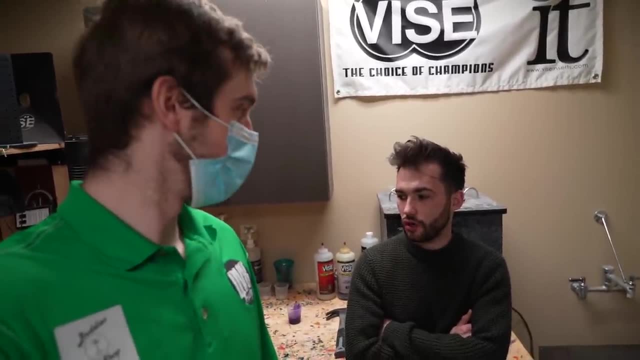 With the hole Three to seven boards more. Probably earlier. Definitely earlier. Definitely earlier. Patrick, 100%. What am I shooting, though? I would say a good score would be about 167 after watching the ball yesterday, But 167.. 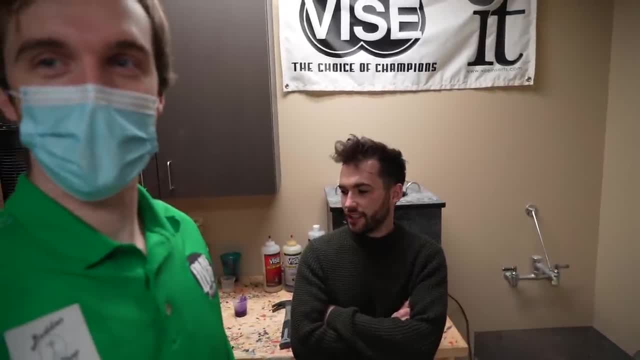 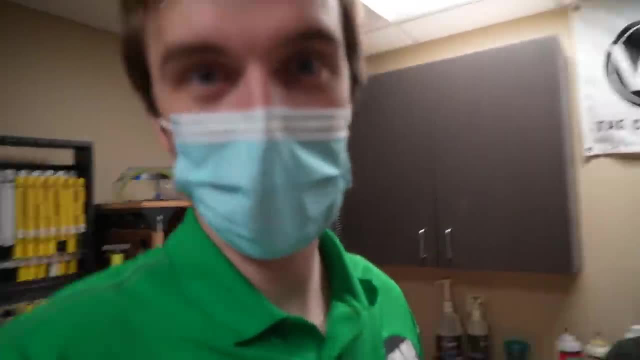 That's on making all my spares. I would say, if I had to be an optimist, I would say about 226.. Out the gate, 226.. If I shoot any less or more than 226,. it's the last video on the channel boys. 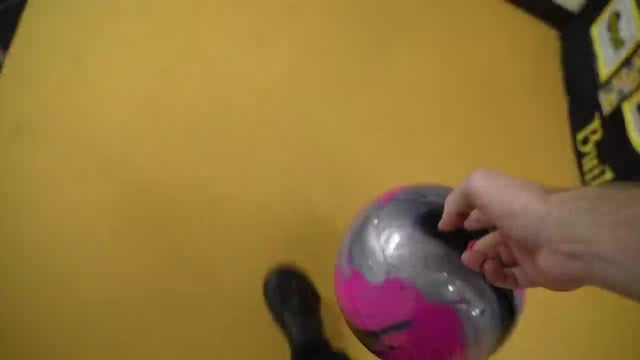 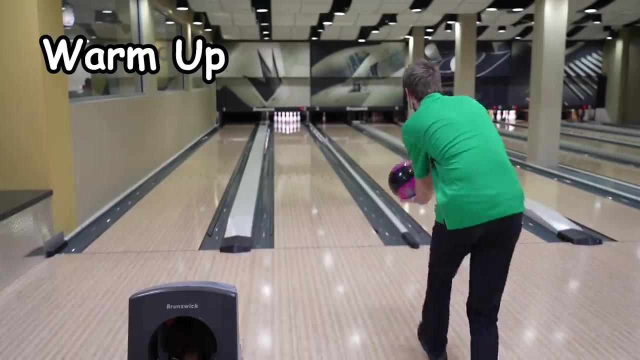 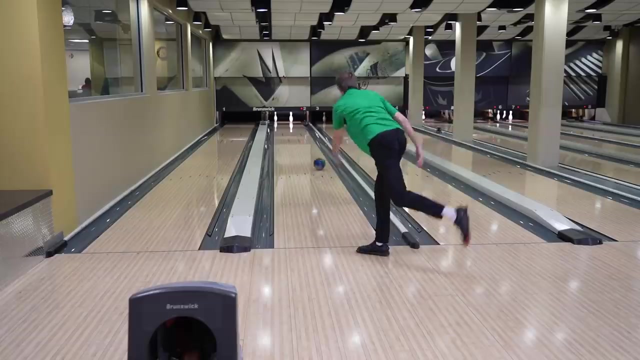 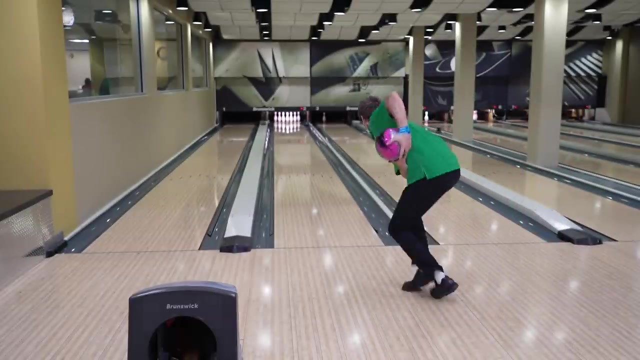 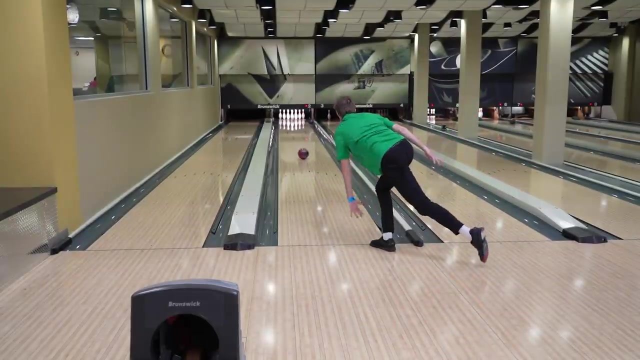 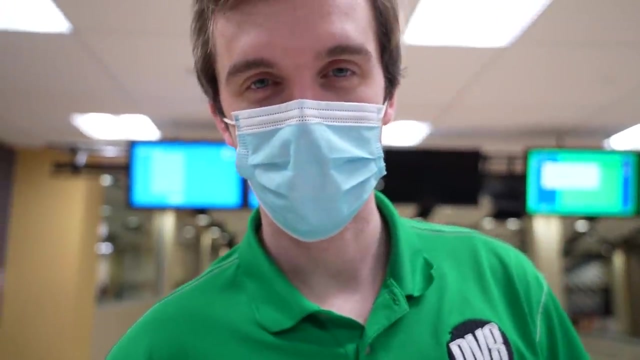 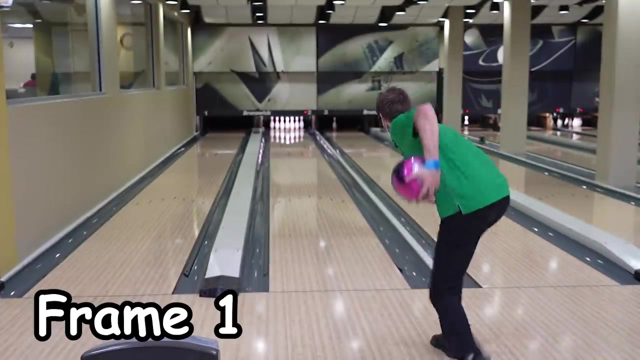 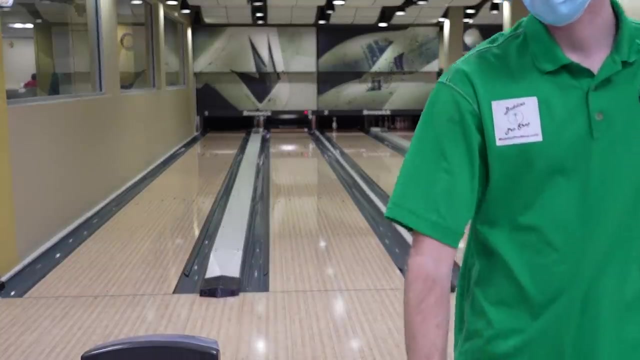 What? Let's get to the lance. All right, Let's go. Sloan lied to me: This ball hooks like three to four less and it hooks way earlier. It kind of bails out downwind. Okay, The ball's actually not bad. it surprised me today. 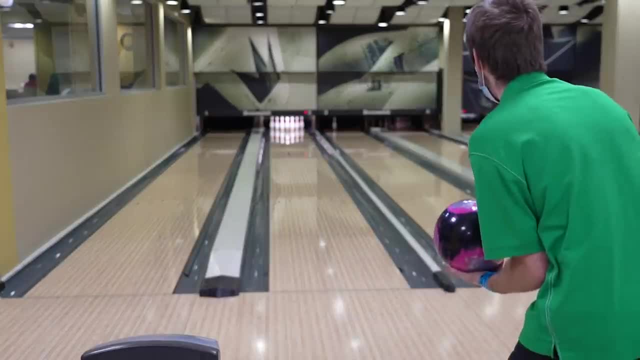 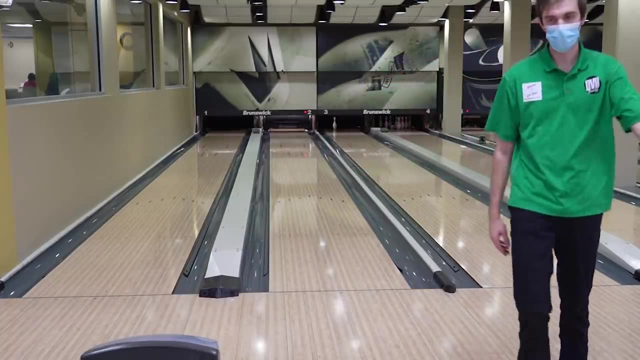 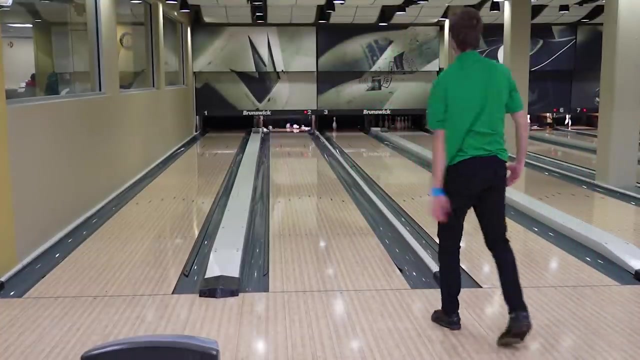 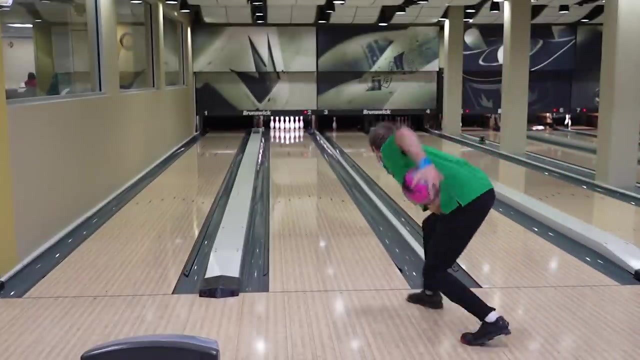 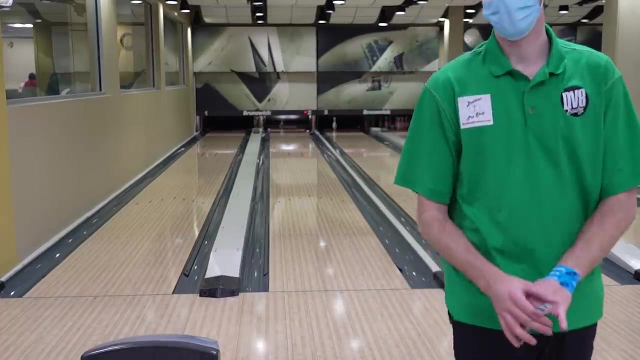 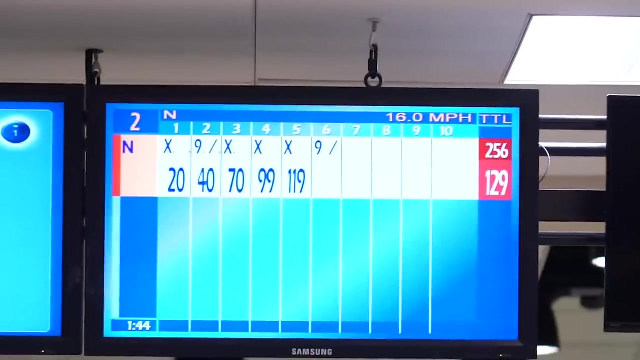 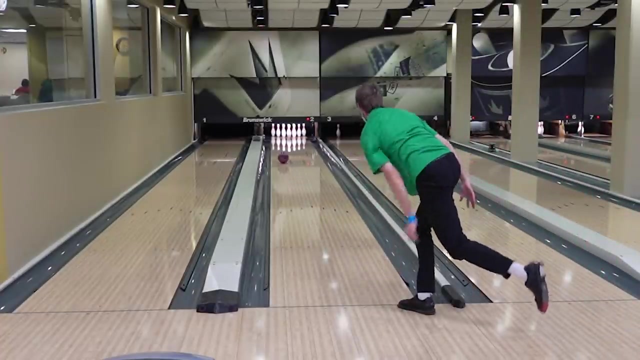 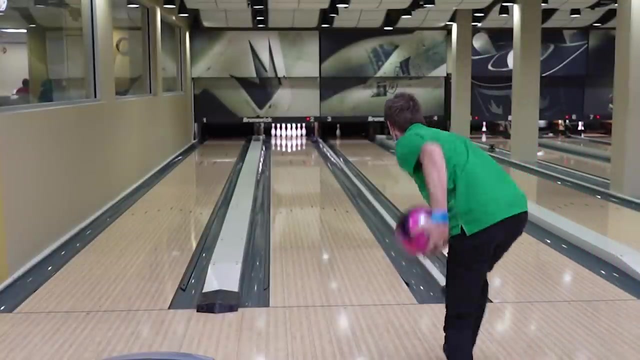 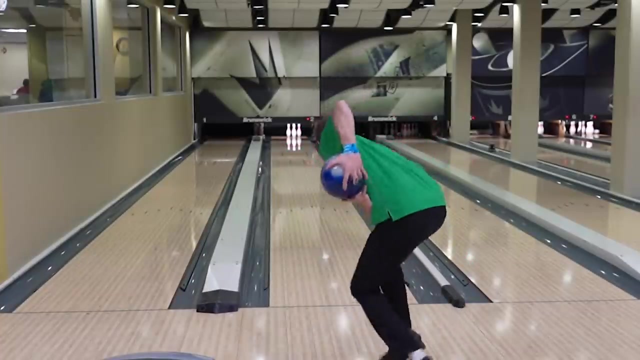 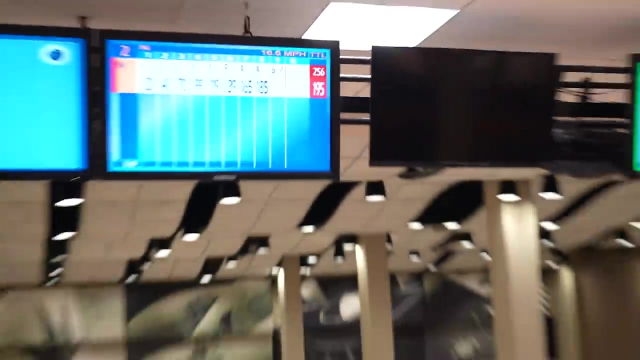 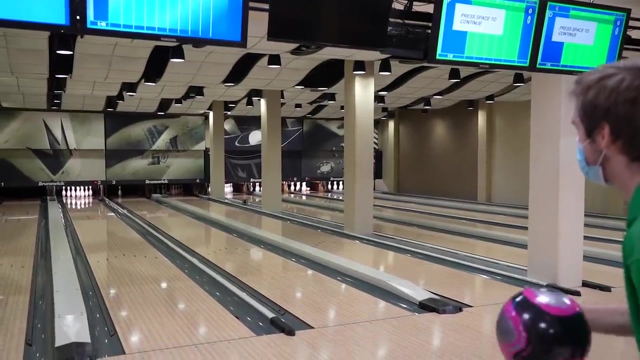 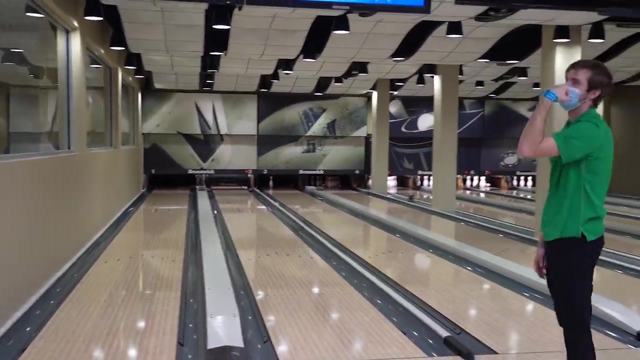 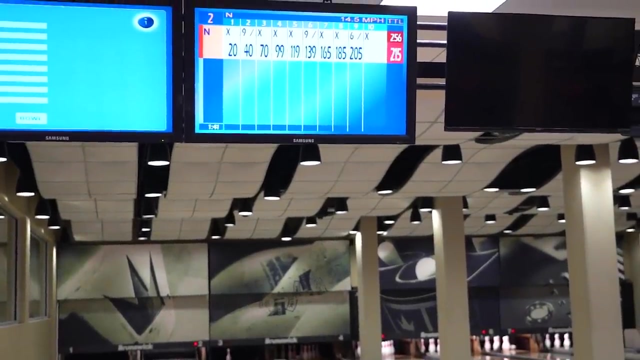 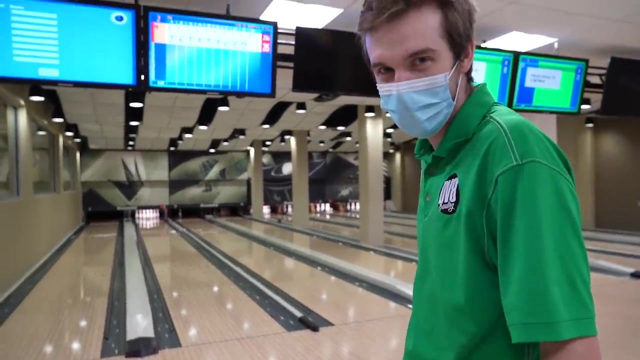 That shot was perfect. I just slapped that thing at the bottom. I've never thrown a better shot in my life. Need a double, need a double. I feel like I completely just screwed myself here. Not only do I need this next one, then I need to get one. 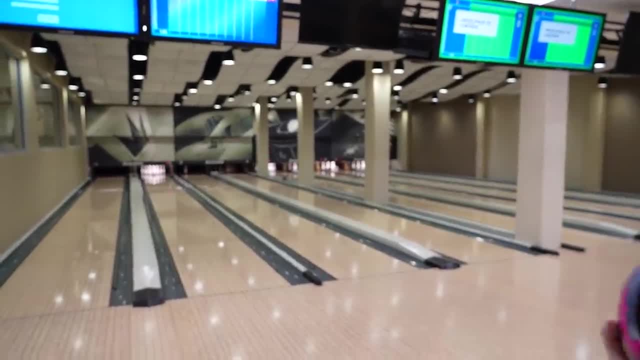 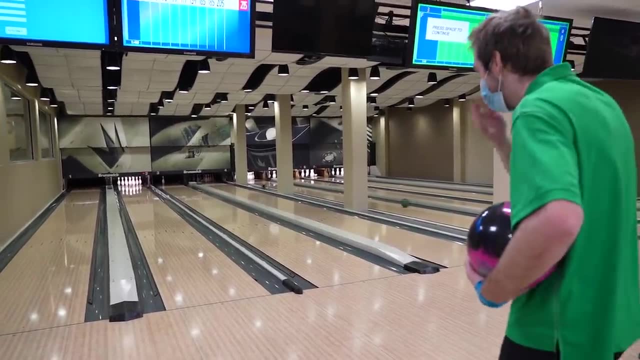 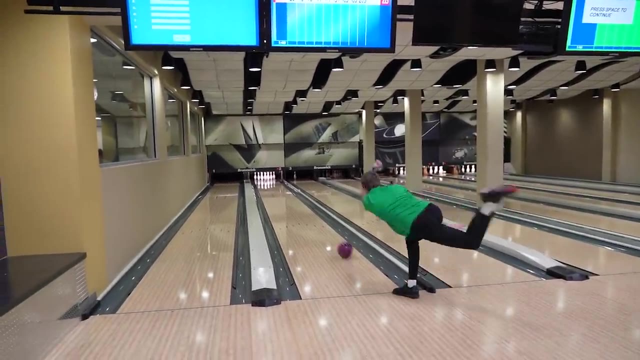 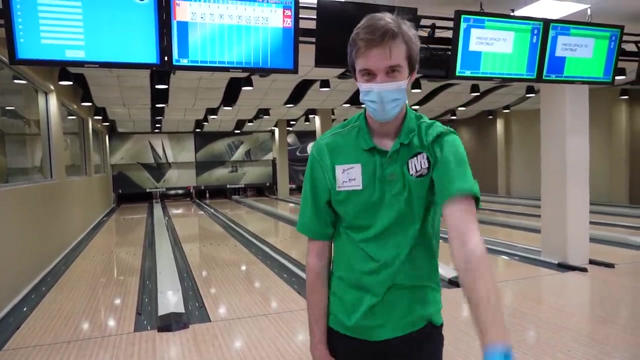 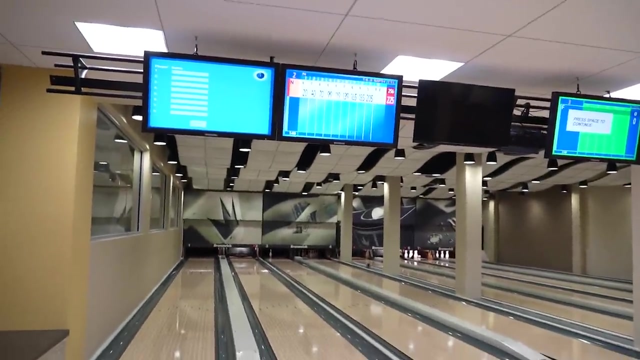 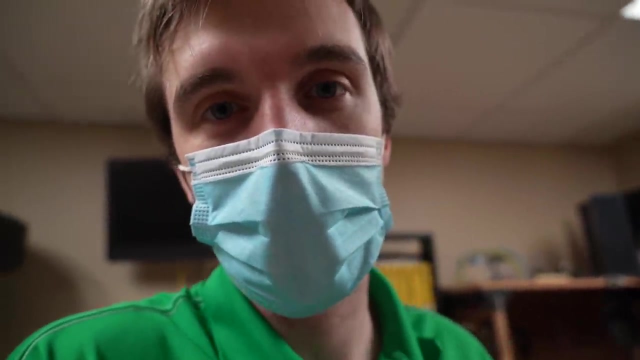 It's a toughie Time to break out the tacky laser pointer. I need one 226.. If I shoot any less or more than 226, it's the last video on the channel boys. Do I go for the 7 or the 10?? 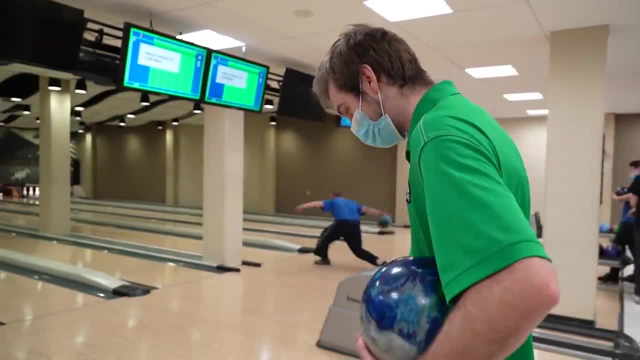 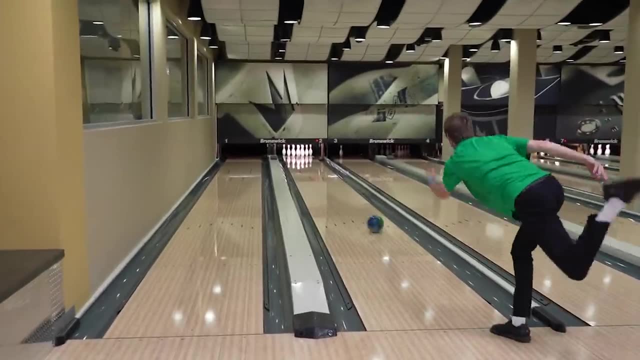 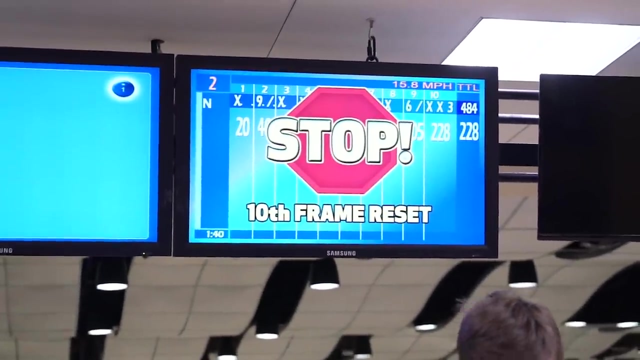 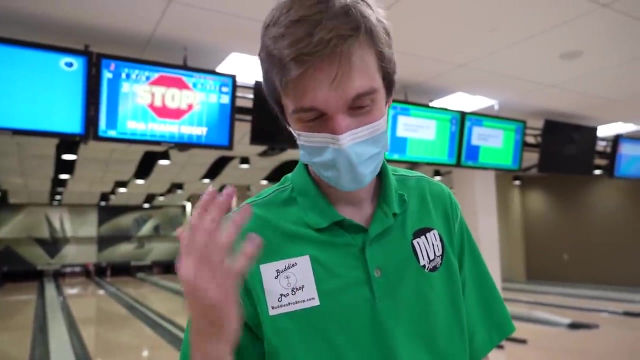 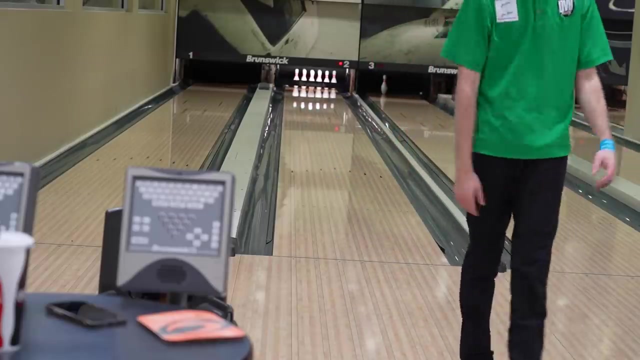 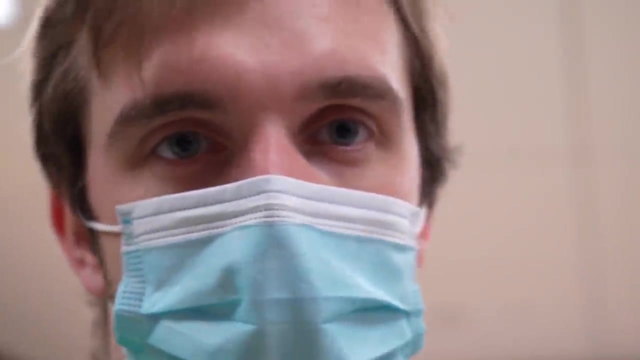 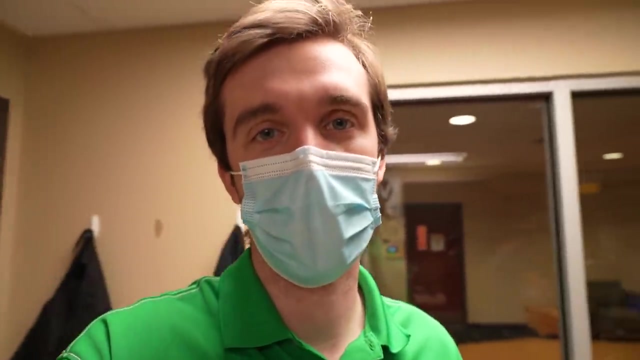 You gotta go for the 7.. Here we go. That was my moment for like a legendary moment on the channel. I got no clutch, all right, well guys, i i did my best- 228, and this is the last video on the channel that you're gonna. 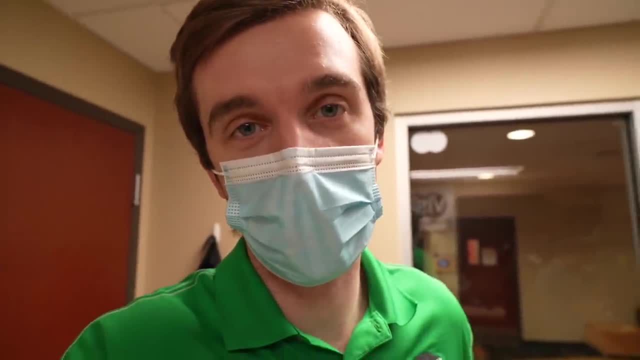 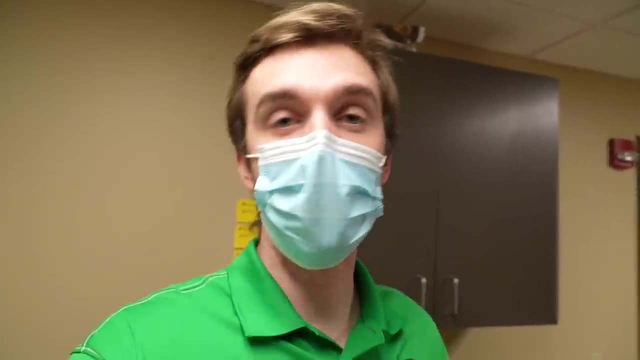 see, because sloan challenged me and i just i wasn't up for it. i got three instead of one. no, clutch, pressure makes diamonds. man, i said pressure makes diamonds. what did you say to me? all right, so, as you guys saw, christopher sloan is an absolute liar, because he told me i was. 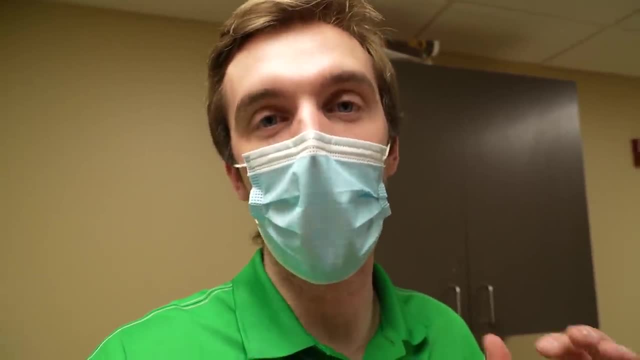 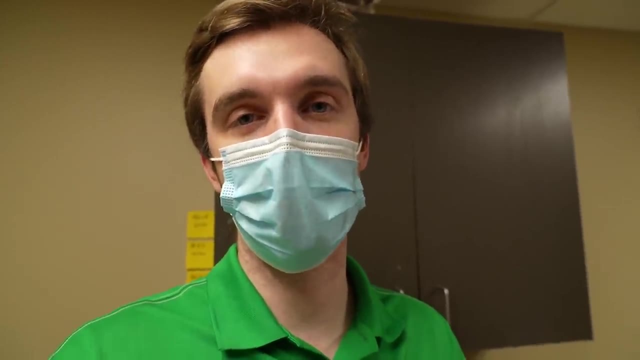 gonna hook three to seven more. it hooked the exact same amount, just in a way different way. so, as you guys saw, with the weight hole it was much slower, it didn't hook quite as much down lane but it gave me a little misroman and honestly it just made it. it made it smoother. 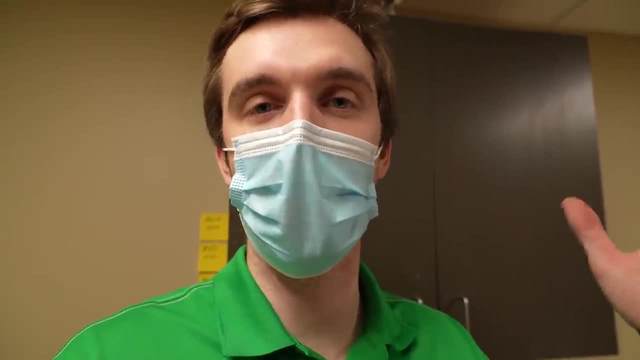 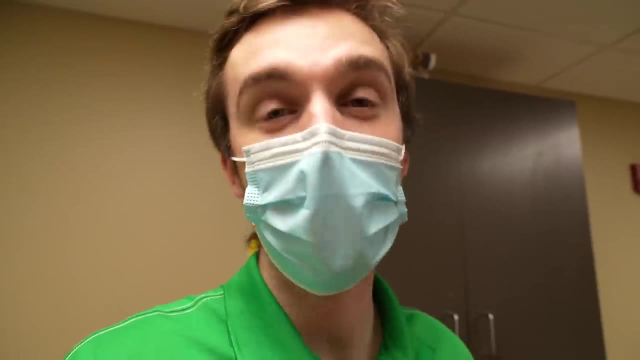 so it made it almost like a hybrid, turned into like a solid type shape down lane. um, so i need to figure out how to drill balls like that, because i loved it. yeah, what i'm telling all you two handers is: christopher sloan is a genius and i'm gonna start laying. 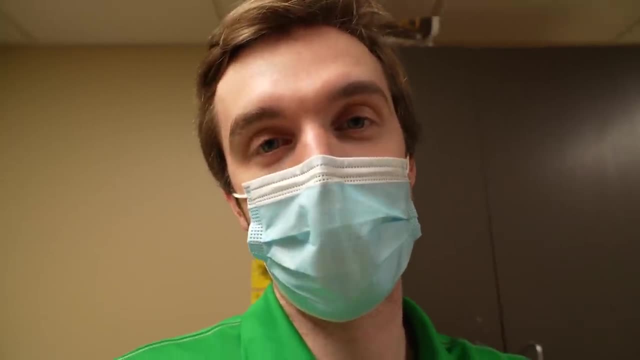 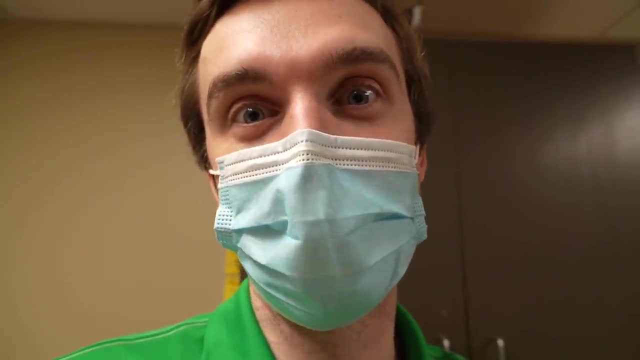 balls out a little smoother because i really like the way that looked. but either way, deviate collision money, pack your spare game, garbage video out.